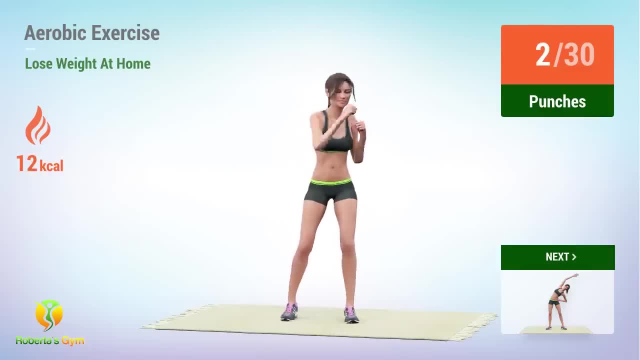 Up next resurrection. Up next punches In 5,, 4,, 3,, 2,, 1, go 1,, 2,, 3,, 4,, 5,, 6,, 7,, 8,, 9,, 10,, 11,, 12,, 13,, 14,, 15,, 16,, 17,, 18,, 19,, 20,, 21,, 22,. 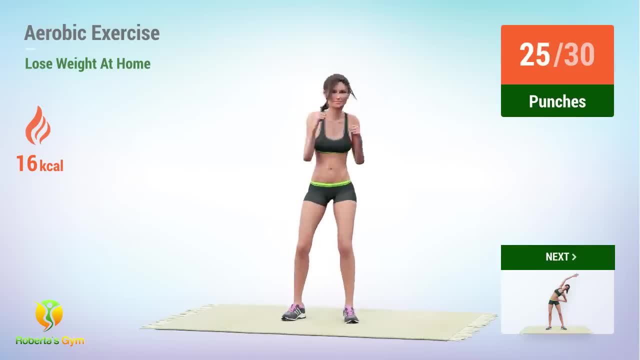 23,, 24,, 25,, 26,, 27,, 28,, 29,, 30.. Up next side bends In: 5,, 4,, 3,, 2, 1, go 1,, 2,, 3,, 4.. 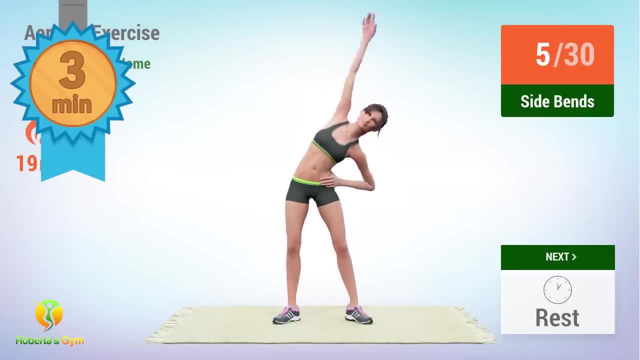 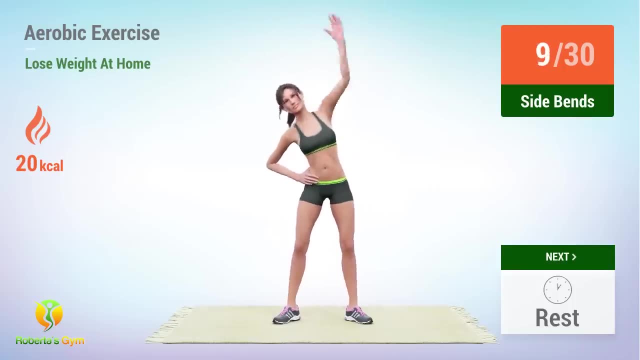 Awesome. You've been exercising for 3 minutes already. Keep going, Don't stop. 8,, 9,, 10,, 11,, 12,, 13,, 14,, 15,, 16,, 17,, 18,. 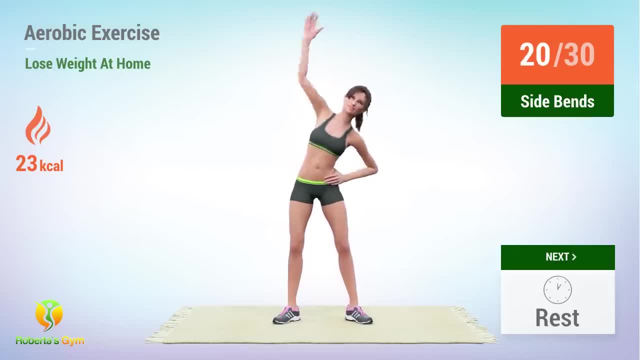 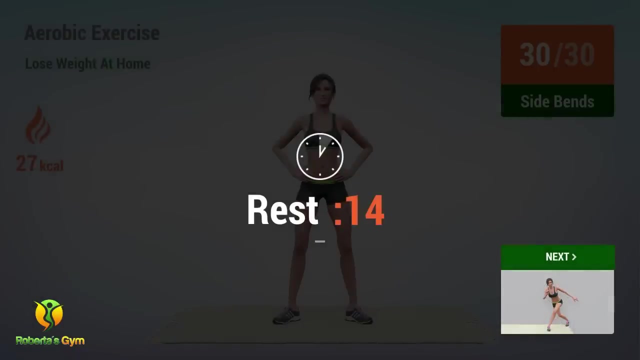 19,, 20,, 21,, 22,, 23,, 24,, 25,, 26,, 27,, 28,, 29,, 30.. Rest time: 10, 9,, 10,, 11,, 12,, 13,, 14,, 15,, 16,, 17,, 18,, 19,, 20,, 21,, 22,, 23,, 24,, 25,, 26,, 27,, 28,, 29,, 30. 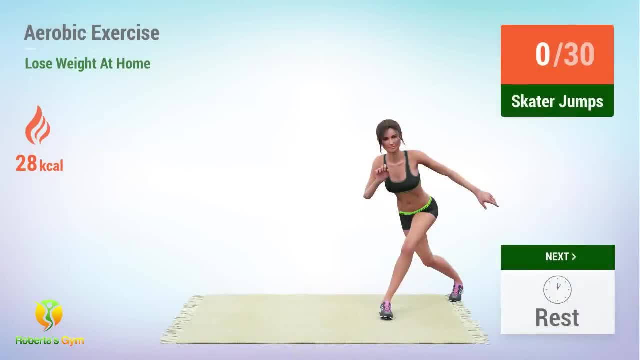 Up. next skater jumps In 5,, 4,, 3,, 2,, 1, go 1,, 2,, 3.. 3,, 4,, 5,, 6,, 7,, 8,, 9,, 10,, 11,, 12,, 13,, 14,, 15,, 16,, 17,, 18,, 19,, 20,, 21,, 22,, 23,, 24,. 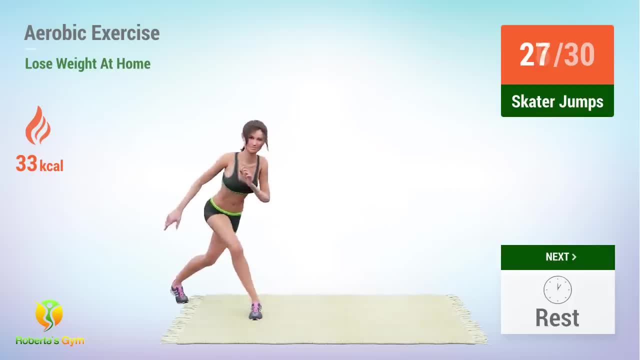 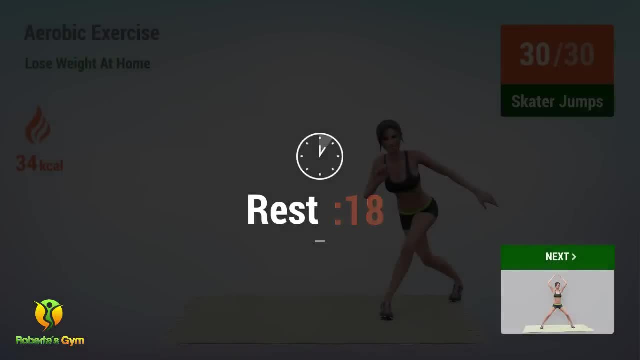 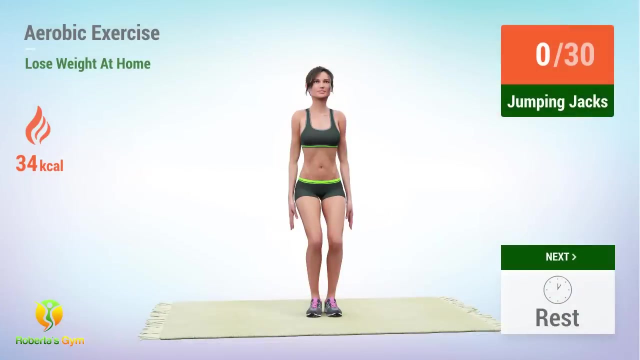 25,, 26,, 27,, 28,, 29,, 30. Rest time- Rest time. Rest time. Up next jumping jacks In 5,, 4,, 3,, 2,, 1, go. 1,, 2,, 3,, 4,, 5,, 6,, 7,, 8,, 9, 10.. 1, 2,, 3,, 4,, 5,, 6,, 7,, 8,, 9, 20.. 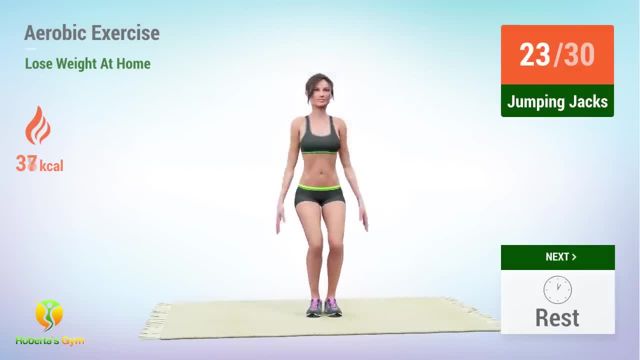 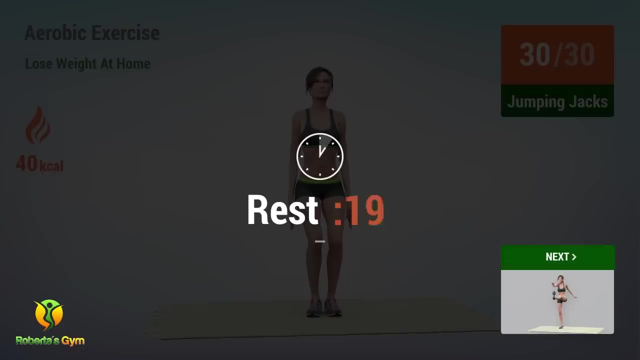 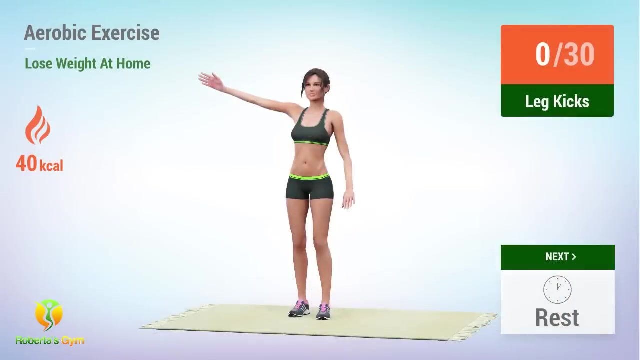 1,, 2,, 3,, 4,, 5,, 6,, 7,, 8,, 9, 30. Rest time: First threw leg kicks Up. next leg kicks In: 5,, 4,, 3,, 2, 1, go. 1,, 2,, 3,, 4,, 5,, 6,, 7,, 8,, 9,, 10,, 21,, 22,, 23,, 24, 25.. 11,, 12,, 13,, 14,, 15,, 16,, 17,, 18,, 19,, 20,, 21,, 22,, 23,, 24,, 25,, 26,, 27,, 28,, 29,, 30. 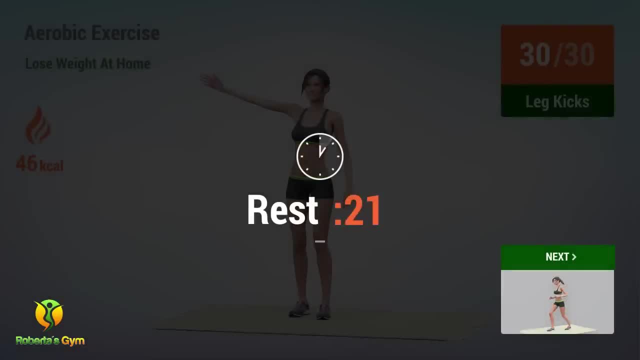 Rest time: 10,, 12,, 13,, 14,, 15,, 16,, 17,, 18,, 19,, 20,, 21,, 22,, 23,, 24,, 25,, 26,, 27,, 28,, 29,, 30.. 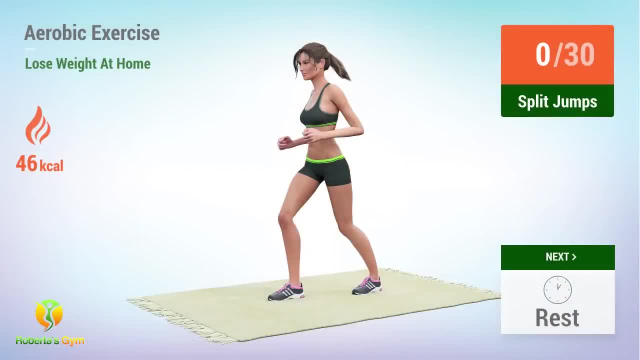 Up. next split jumps In 5,, 4,, 3,, 2,, 1.. Go 1,, 2,, 3,, 4,, 5,, 6,, 7,, 8,, 9,, 10,, 11,, 12,, 13,, 14,, 15,, 16,, 17,, 18,, 19,, 20,, 21,, 22,, 23,, 24,, 25,, 26,, 27,, 28,, 29,, 30. 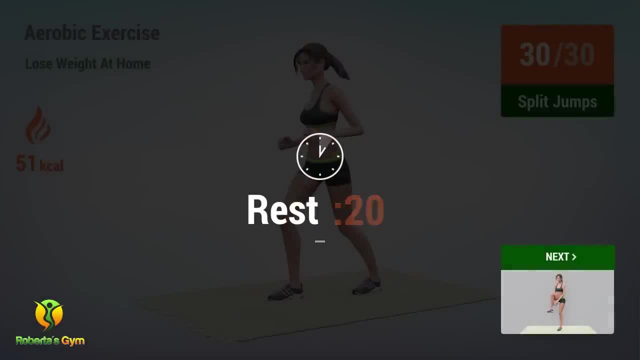 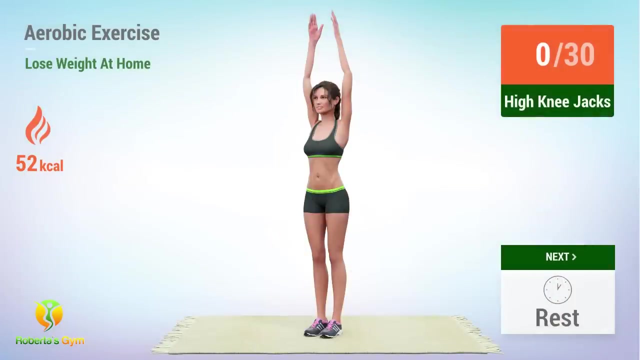 Rest time. Up next high knee jacks. Up next high knee jacks. Up next high knee jacks In: 5, 4,, 3,, 2, 1. Go 5, 4, 3,, 2,, 1, go. 1,, 2,, 3,, 4,, 5,, 6,, 7,, 8,, 9,, 10,, 11,, 12,, 13,, 14,, 15,, 16,, 17,, 18,, 19,, 20, 21.. 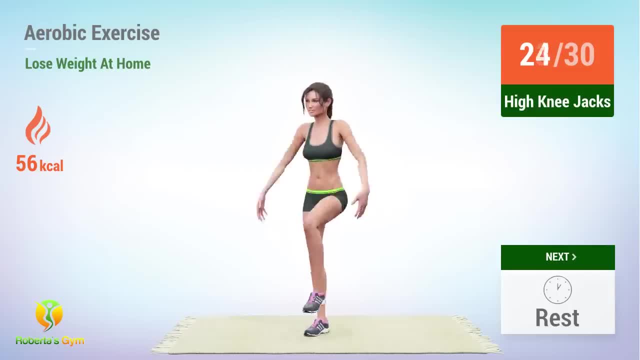 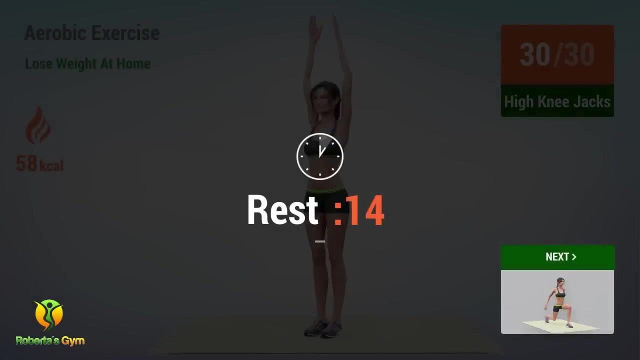 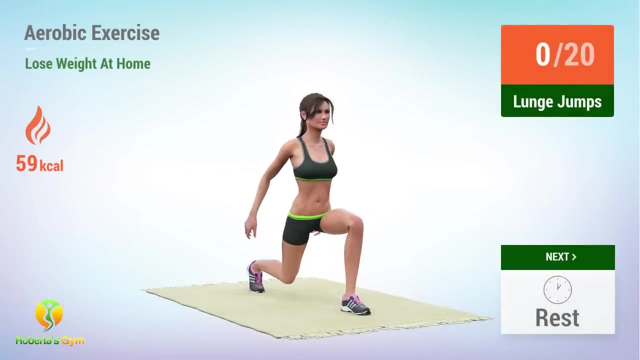 22,, 23,, 24,, 25,, 26,, 27,, 28,, 29,, 30. Rest time. Up next lunge jumps In 5,, 4,, 3,, 2, 1, go. 1,, 2,, 3,, 4,, 5,, 6,, 7,, 8,, 9,, 10,, 11,, 12,, 13,, 14,, 15,, 16,, 17,, 18,, 19, 20.. 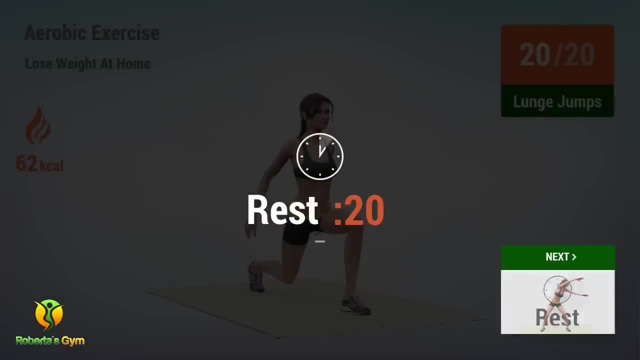 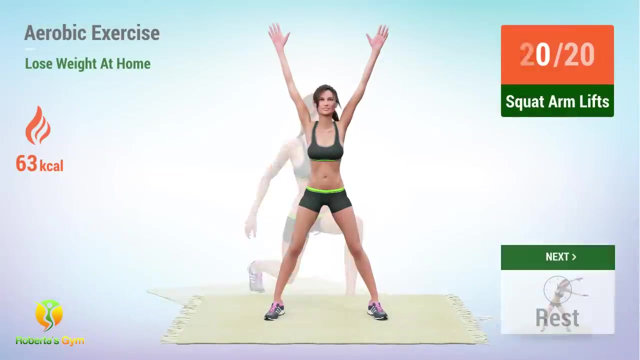 Up next lunge jumps: 17,, 18,, 19,, 20.. Rest time: Up next squat arm lifts In 5, 4, 3, 2, 1, go In 5, 4, 3, 2, 1, go. 1,, 2,, 3,, 4,, 5,, 6,, 7,, 8,, 9,, 10,, 11,, 12,, 13,, 14,, 15,, 16,, 17,, 18,, 19, 20.. 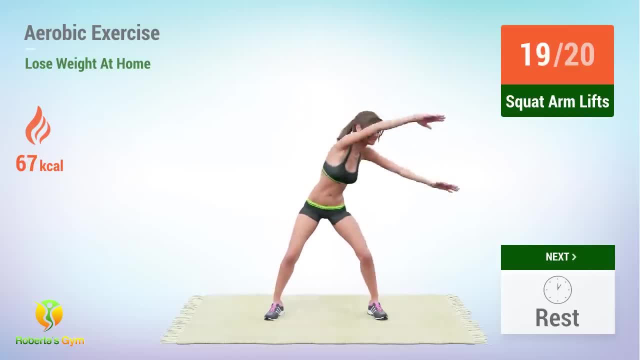 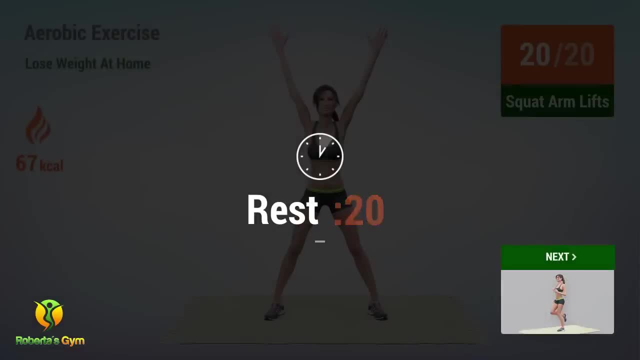 Rest time. Up next lunge jumps In 5,, 4,, 3,, 2, 1, go, 1, 2,, 3,, 2, 1, go Rest time- Rest time. 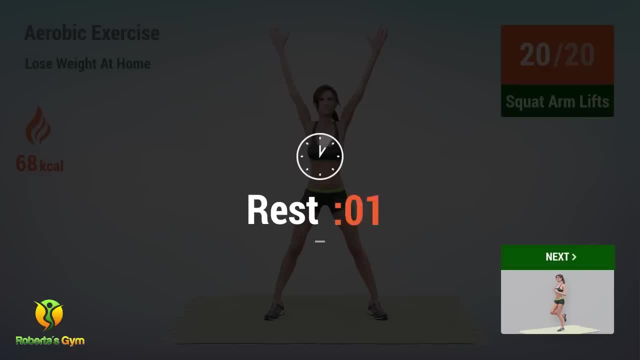 In 5,, 4,, 3,, 2, 1, go 1, 2, 3, 2, 1, go. 17,, 18,, 19, 20.. Rest time Up next running in place. 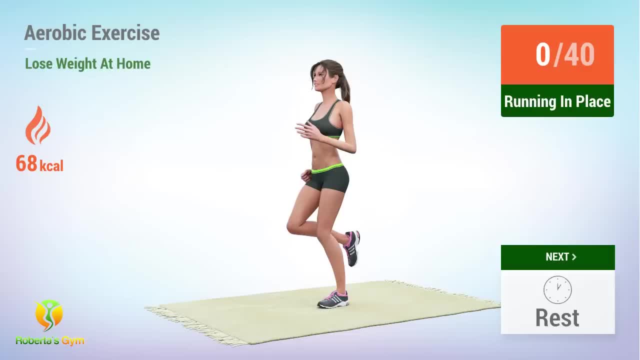 In 5,, 4,, 3,, 2,, 1, go 2,, 4,, 6,, 8,, 10,, 12,, 14,, 16,, 18,, 20,, 22,, 24,, 26,, 28,, 30,, 32,, 34,. 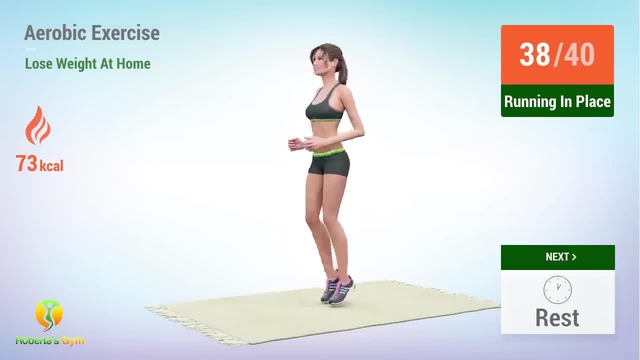 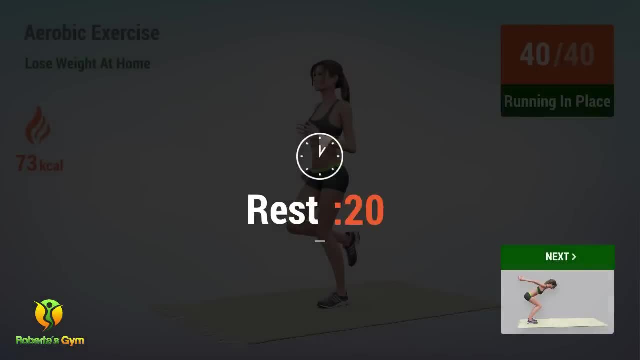 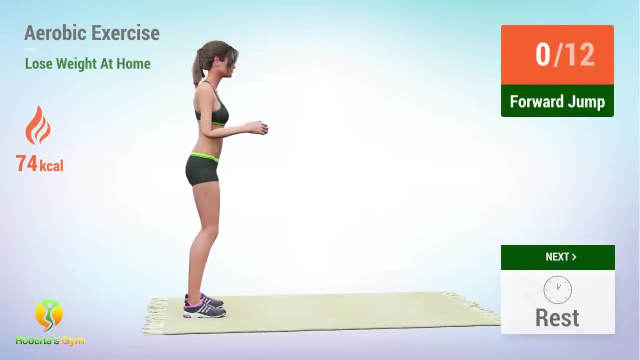 35,, 36,, 37,, 38,, 39,, 40, 36,, 38,, 40, rest time. Up next four jump In 5,, 4,, 3,, 2,, 1, go. 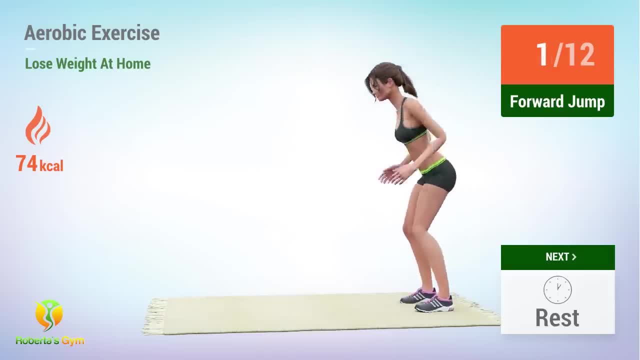 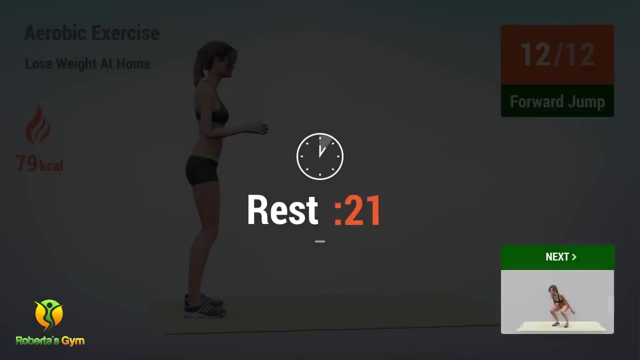 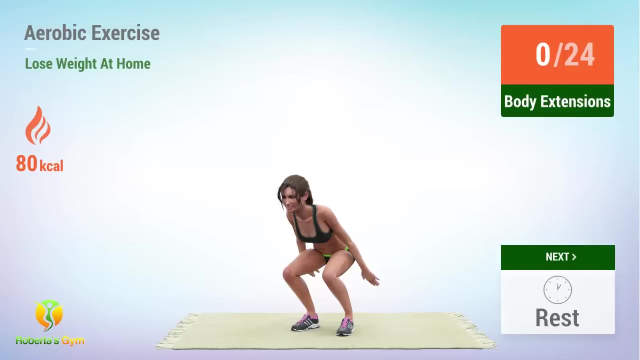 1,, 2,, 3,, 4,, 5,, 6,, 7,, 8,, 9,, 10,, 11,, 12, rest time. Up next body extensions In 5,, 4,, 3,, 2,, 1, go. 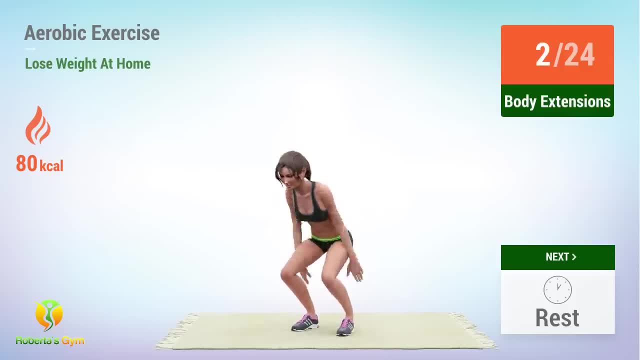 1,, 2,, 3,, 4,, 5,, 6,, 7,, 8,, 9,, 10,, 11,, 12,, 13,, 14,, 15,, 16,, 17,, 18,, 19,, 20,, 21,, 22,, 23,, 24, rest time. 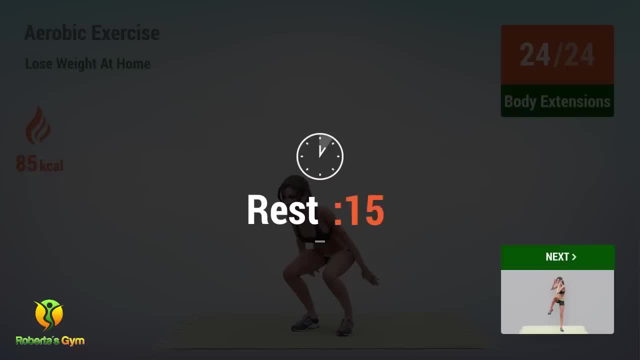 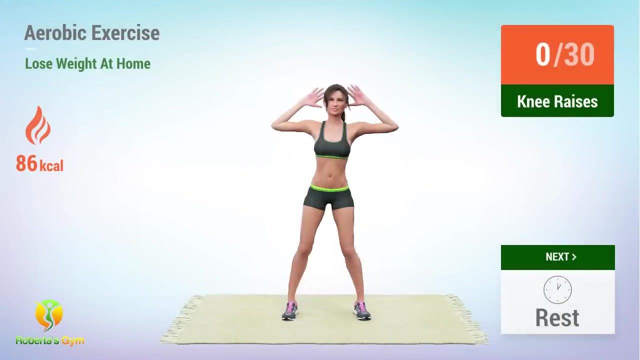 Up next knee raises In 5,, 4,, 3,, 2,, 1, go 1,, 2,, 3,, 4,, 5,, 6,, 7,, 8,, 9,, 10,, 12,, 13,, 14,, 15,, 16,, 17,, 18,, 19,, 20,, 21,, 22,, 23,, 24, rest time. 1,, 2,, 3,, 4,, 5,, 6,, 7,, 8,, 9,, 10,, 11,, 12,, 13,, 14,, 15,, 16,, 17,, 18,, 19,, 20,, 21,, 22,, 23,, 24,, 25,, 26,, 27,, 28,, 29,, 30,, 35,, 36,, 37,, 38,, 39,, 40.